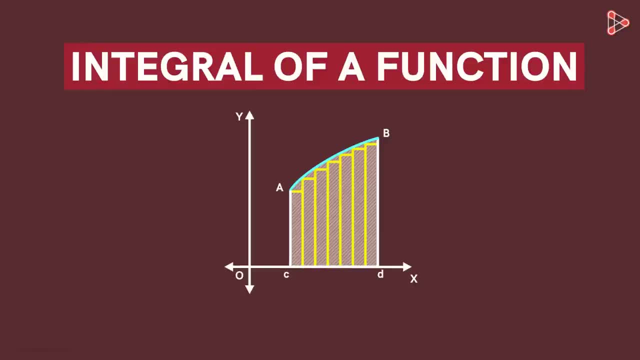 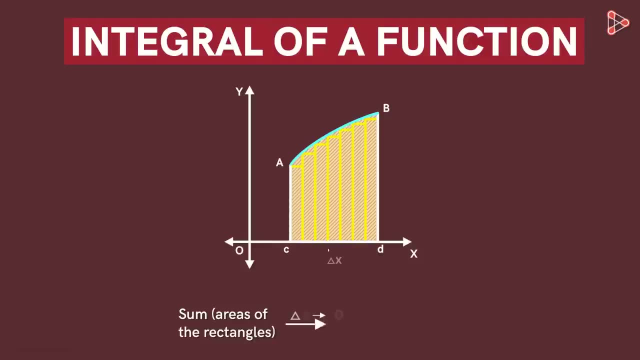 First we divide the area into rectangles, Then we find the sum of the areas of the rectangles. Then, to get the area under the graph, we take the limit of the sum of the areas. as the width of the rectangles tends to zero, We can see that this process is a bit lengthy and cumbersome. 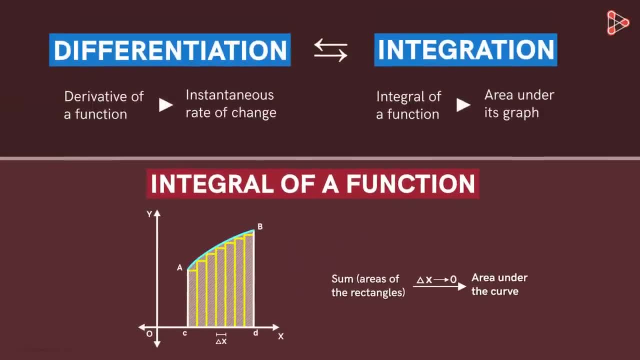 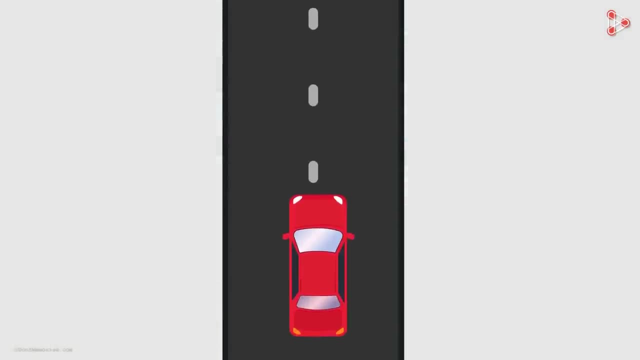 We can't do this every time, So now we will see that this relation comes to our rescue. It gives us an easier way of finding the integral of the function. So let's get started. Let's say that we are travelling on a road. 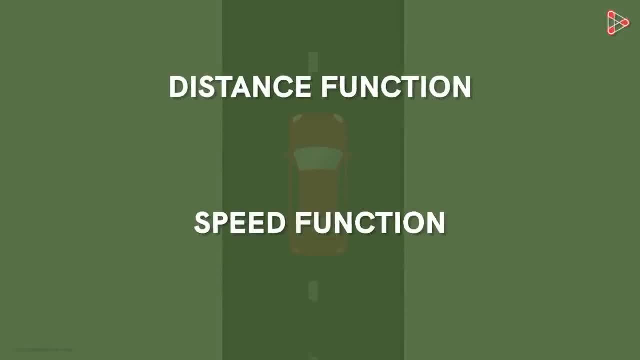 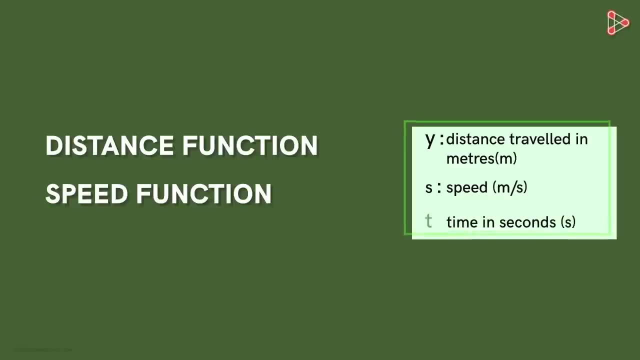 We know that the distance travelled by the car and its speed are both functions of time. Let's denote the distance travelled with variable y and the speed with s and the time elapsed with t. Now suppose the distance travelled by the car is this function of time. 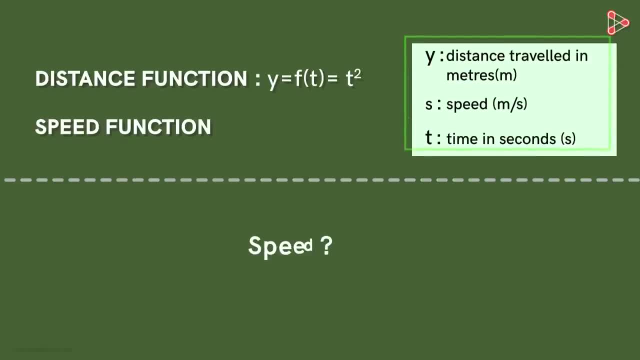 It's the square of t. Can you tell me what will be the speed of the car at any instant t? The speed at an instant t is the instantaneous rate of change of the distance travelled, So it will be equal to the derivative of the distance function at the instant t. 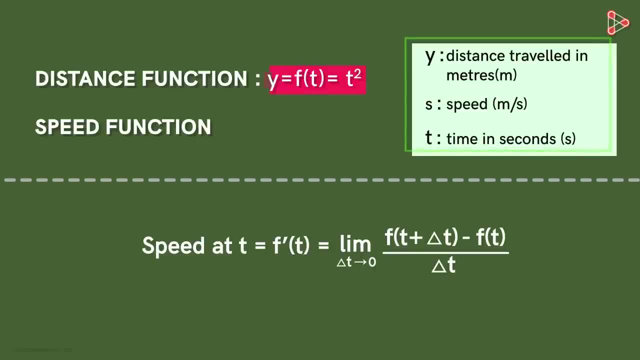 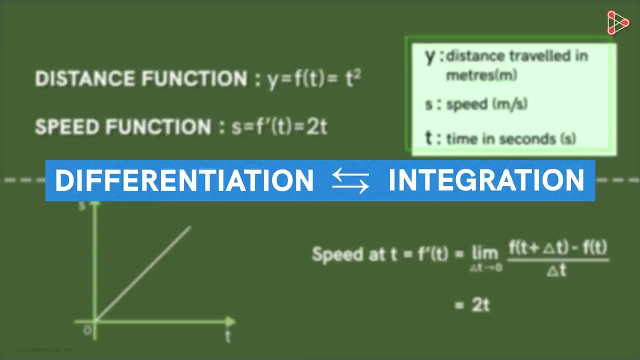 And we have seen earlier that the derivative of this function is equal to two times t. So this function will give us the speed of the car at time. t Its graph will look like this: Now, to see the relation between differentiation and integration, consider this integral of the speed function. 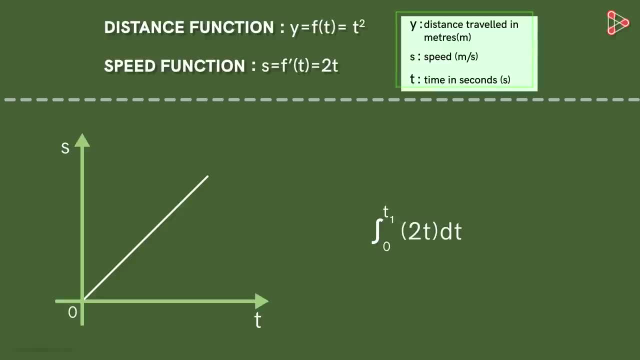 Here. t1 is some arbitrary time instant. Let's mark it here. on this axis, Can you find the value of this integral? For this we need to find this area under the graph, But since this is a triangle, we don't even have to use integration here. 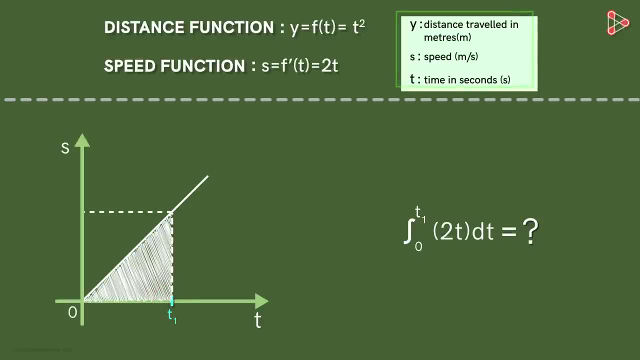 Notice that at t1, the value of this function is equal to two times t1.. So the base of this triangle will be equal to t1 and its height will be equal to two times t1.. So the area of this triangle will be equal to t1 squared. 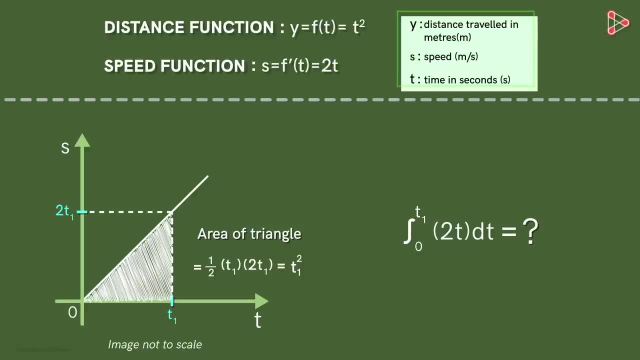 So we get that this integral from zero to t1 is equal to t1 squared. But notice that, according to this distance function, t1 squared is exactly the distance travelled in time: t1.. So what does this tell us? We see that the area under this graph tells us the distance travelled by the car. 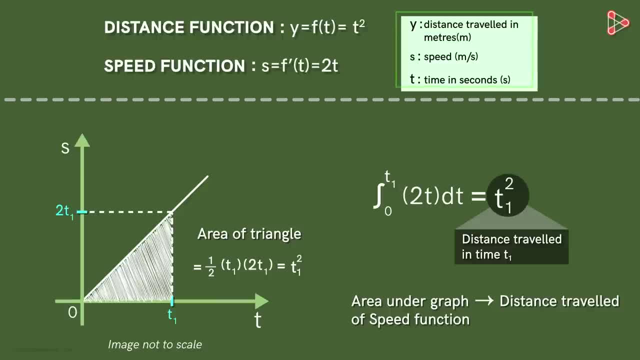 Since t1 is an arbitrary value of time t, this is true for any time, instant t. So this integral is the function of time. This is the connection between integration and differentiation. We have a function f of t and its differentiation gives us this function. 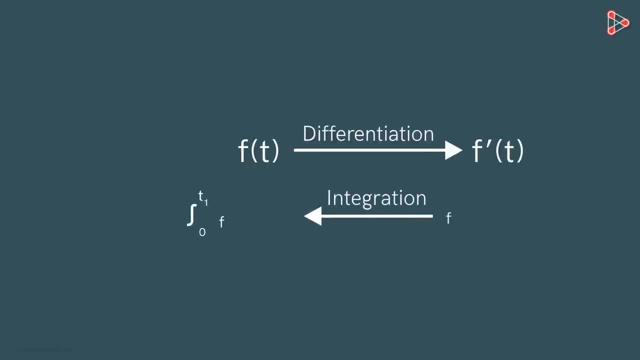 f, prime of t. Now, integration of this derived function gives us the function f of t back. So we see that the process of integration and differentiation act opposite to each other. Integration is the reverse of differentiation And differentiation is the reverse of integration. 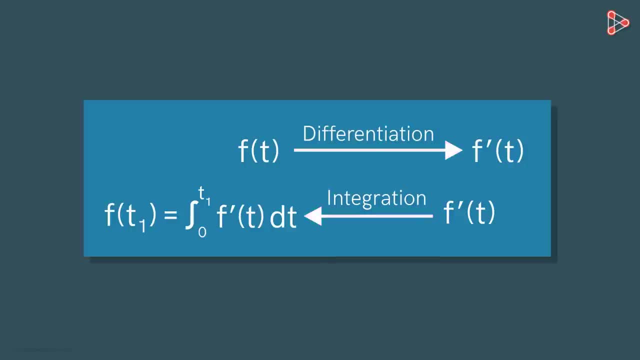 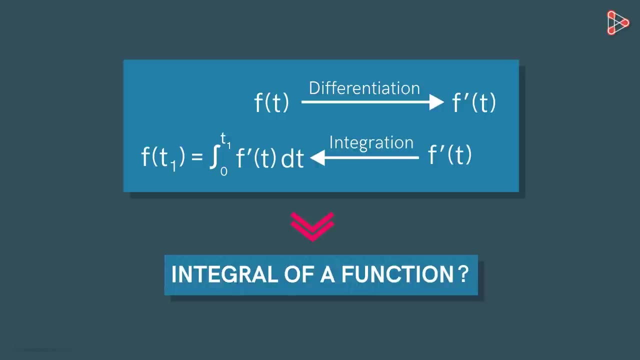 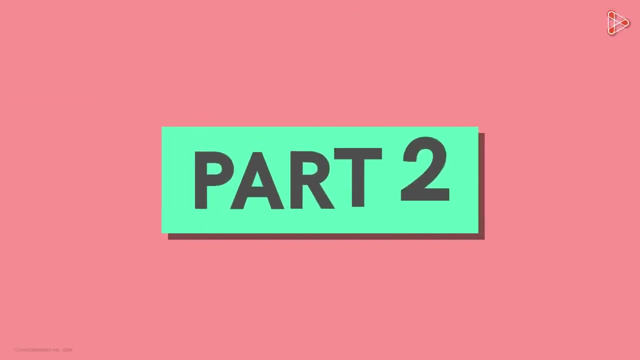 If you remember, we mentioned earlier that this relation can be used to find the integral of the function easily. Can you think of how we can use the following relation for this? Let's see that in the next part. Now we understand that the process of integration 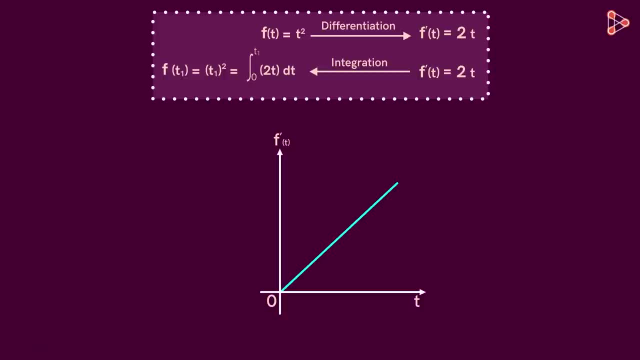 is actually the reverse of differentiation. If we take the integral of the derivative of the function f of t, we get back the function f of t. Take a moment and understand this. Observe this integral. It tells us that for each value of t1,, 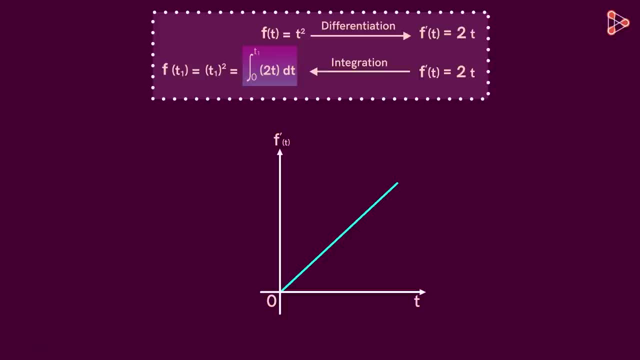 this integral will be equal to the value of the function f of t at t1.. For an arbitrary time, t1, it's equal to this area under the graph. Now let's see how this relation helps us in finding an integral of a function. 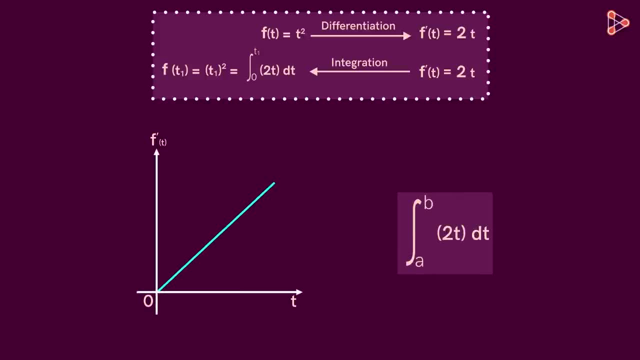 Consider this integral of the function 2t between t equal to a and b. Here a and b are just some constant numbers, Let's say they are these numbers on the t-axis. So this integral will be equal to this area under the graph. 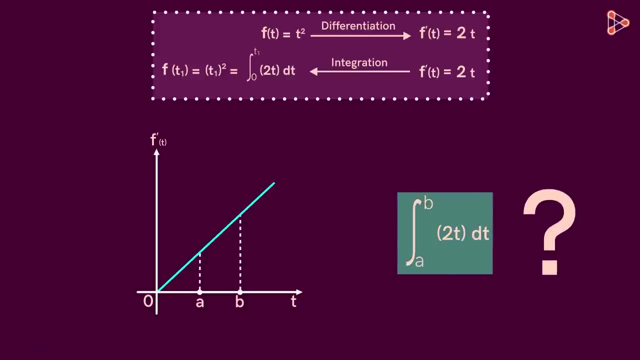 Now, can you tell me what will be the value of this integral? Notice that this area is equal to the difference in the areas between this triangle and this one. Yes, the big triangle minus this small one. We know that the area of this big triangle. 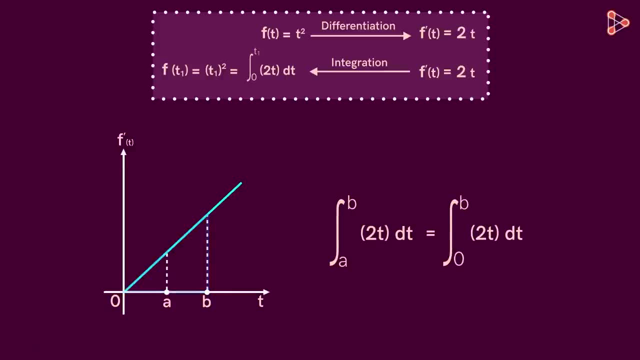 is equal to this integral from zero to b, And the area of this triangle is equal to this integral from zero to a. But now, according to this, we don't have to find the value of these integrals. Notice, these integrals will be equal to this integral. 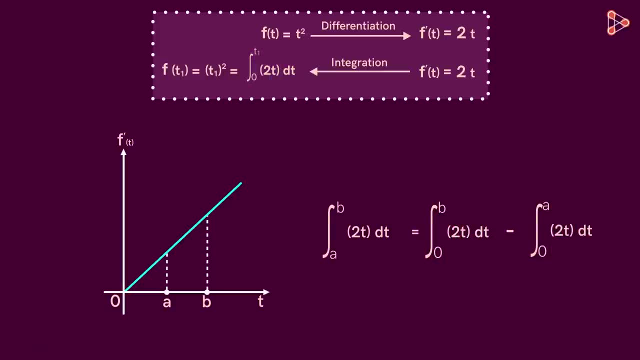 for t1 equal to a and b. So we get the value of this integral is equal to f of b minus f of a. What will this be equal to now? Yes, b squared minus a squared. So we see that using the function f of t. 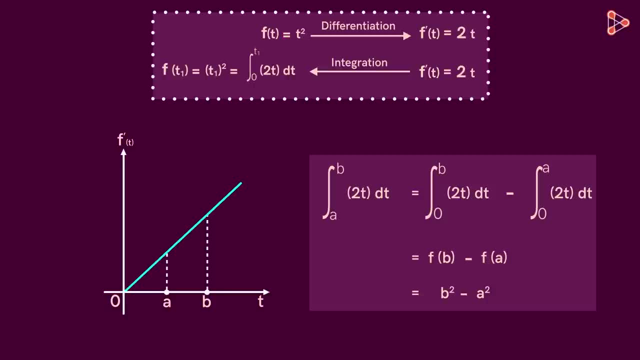 we can easily find any integral of the function, f. prime of t. Any integral of the derivative of the function will be equal to the difference in the value of the function evaluated at the limits of integration. This result is true in general and it's called: 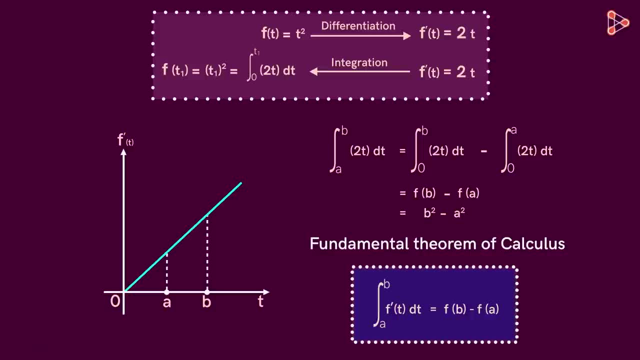 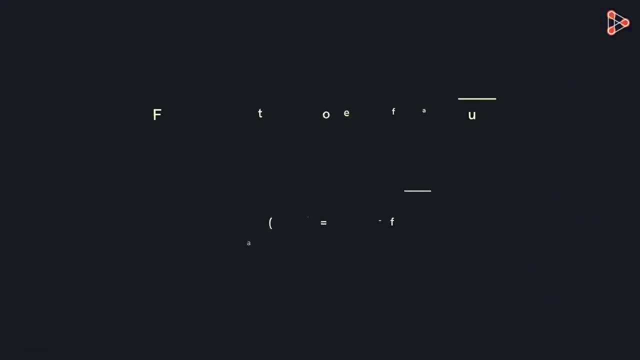 the fundamental theorem of calculus. Now we can use this result to find the integral of a function. Let's see how. So we know the fundamental theorem of calculus. Now consider this function: g of x equal to x squared. Let's say we want to find the integral of this function. 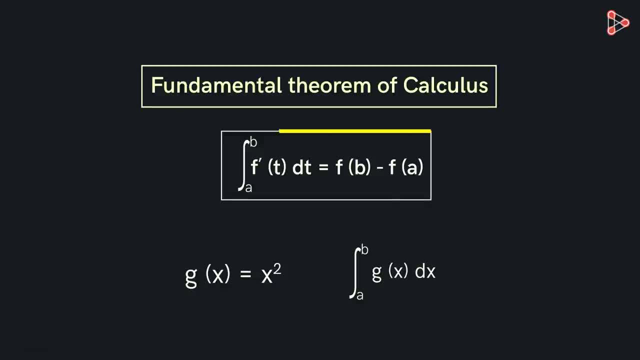 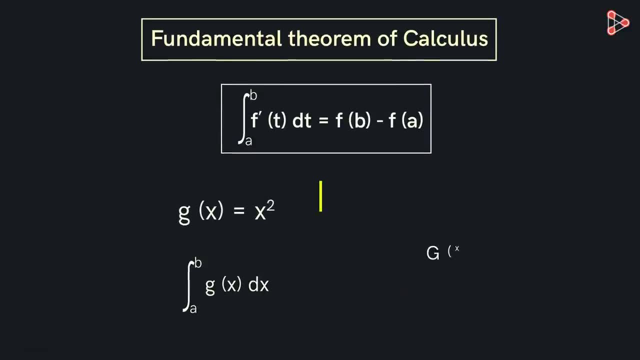 from a to b. Can you tell me how we can use this result to find this integral? Suppose we find a function- capital G of x- such that its derivative is equal to the function g of x. Since we get that the derivative of capital G of x? 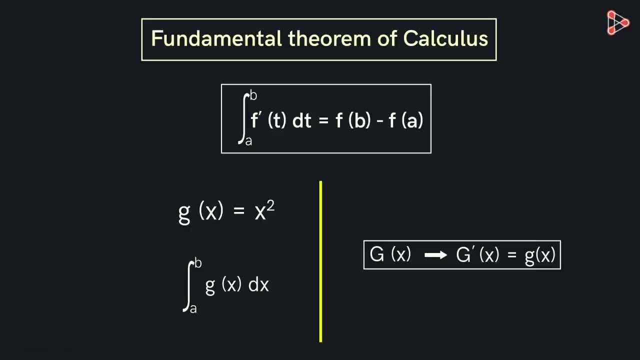 is equal to g of x, we can see that the integral of this function will be equal to this integral. Now notice that we can apply this result here. We will get the integral of g of x to be equal to capital G of b minus capital G of a.